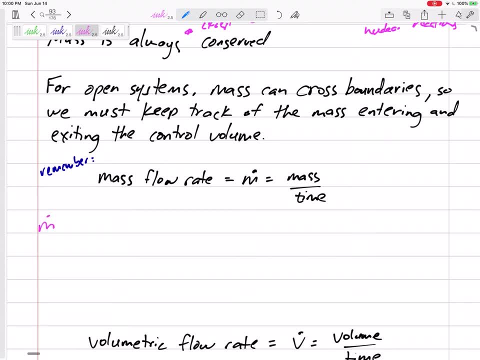 flow rate is mass divided by time. If we have a, let's think about a circular, let's think about a cylinder, Let's think about a tube. If we have a circular inlet or outlet, then the mass flowing through here maybe it's uniform. It probably isn't really uniform, but we could find the 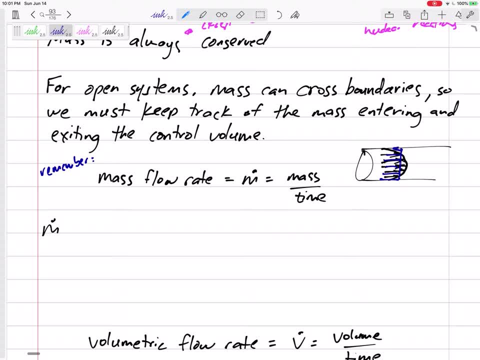 average velocity. We could find the average velocity. The average would technically be something like one over the cross-sectional area times the normal velocity integrated over that cross-sectional area. We won't have to do that, But if we know the average velocity of the inlet outlet. 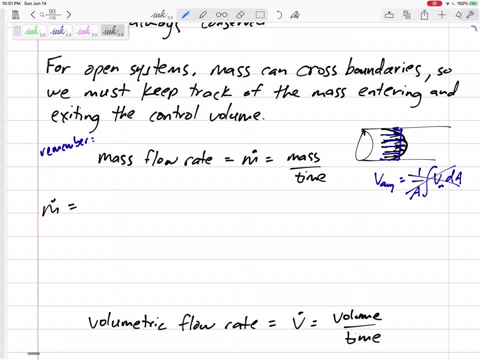 then the mass flow rate will be rho V A. Technically it might be like the integral of rho V, normal D A, you know, V, the velocity that is perpendicular to the cross-sectional area. Again, we're probably not going to need. 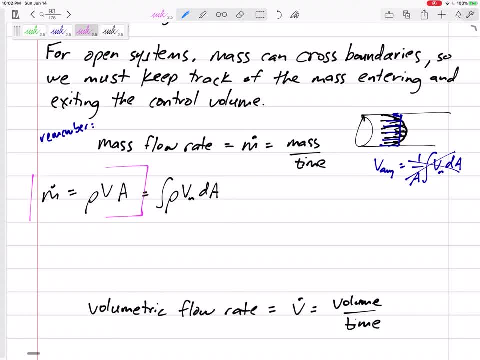 to do that. So let's say m dot is rho, V A, where rho is the density of the fluid, V is the velocity of the fluid. This would be the average velocity of the fluid. This would be the velocity normal to the cross-sectional area, which just means you know the velocity. 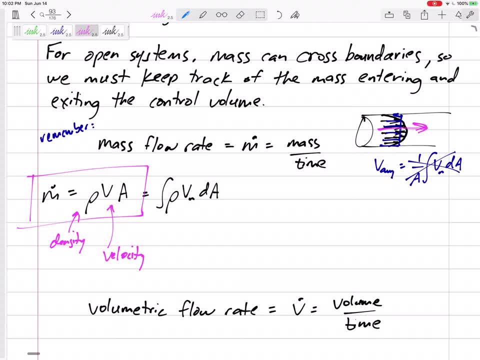 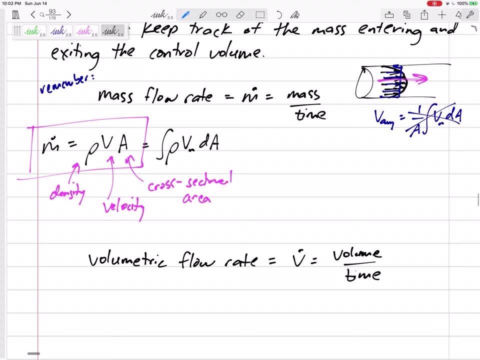 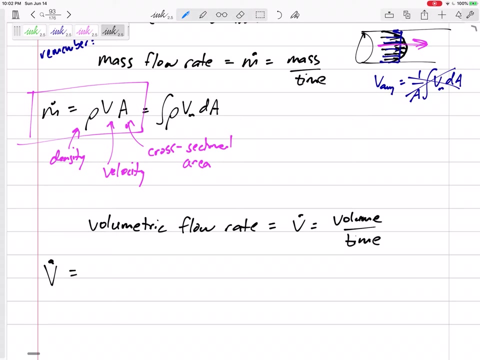 in the direction of the pipe or the inlet, And A is the cross-sectional area. Cross-sectional area- Now don't get it confused with the volumetric flow rate- how much volume we've got per unit time. So maybe if we want volume or we know volume, volumetric flow rate is: 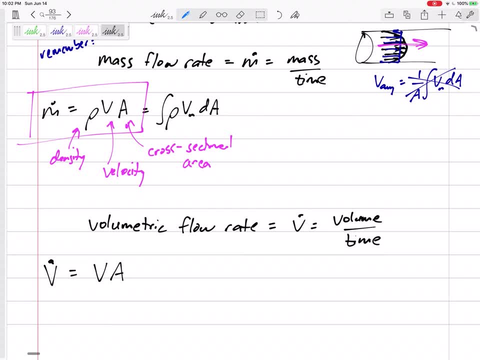 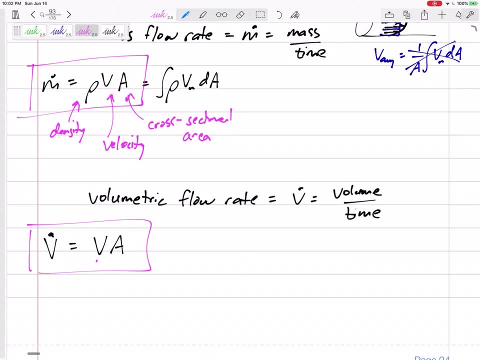 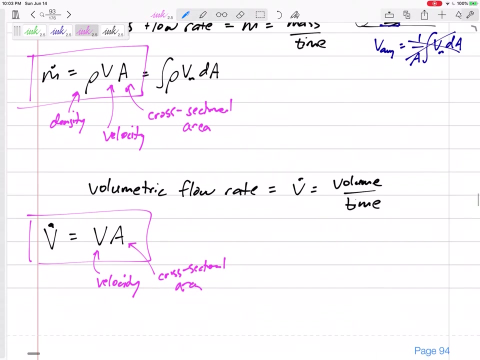 this is V times area where, let's say, this is volumetric flow rate. I think that's obvious. This is velocity, But again, it's really the normal velocity in the direction that it is flowing And A is the cross-sectional area. Technically, this you know. if this is not, 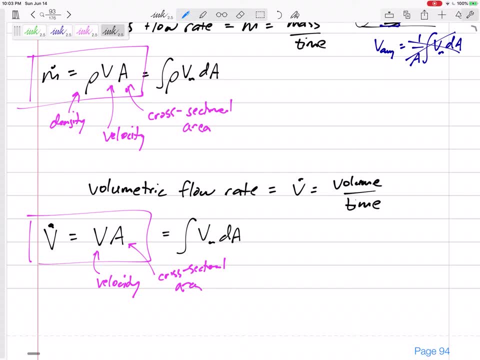 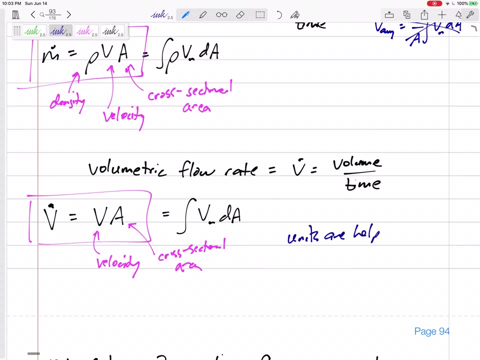 constant. it's really V, V, normal, D, A, as A goes from the whole cross-sectional area. Units are helpful. I've already had it right here. Units are helpful, Right, If we've got kilograms per second right kilograms. 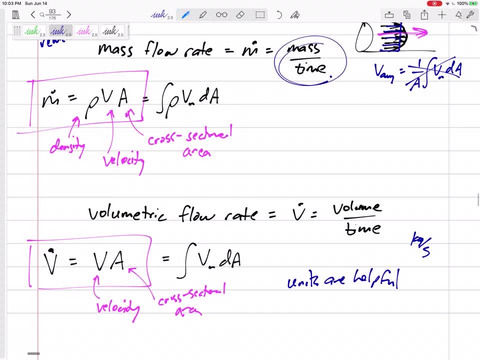 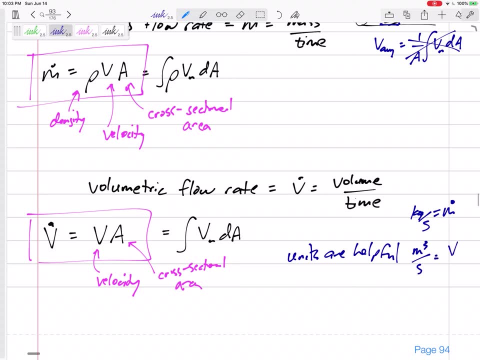 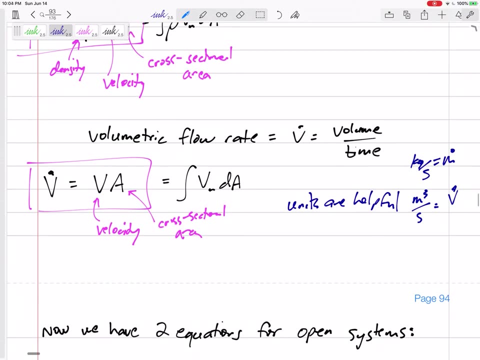 per second, that's volumetric flow rate. right, Right, That is m dot. If we've got something like meters cubed per second, that's V dot, That's volumetric flow rate, All right, And then to kind of switch between the two, maybe you're. 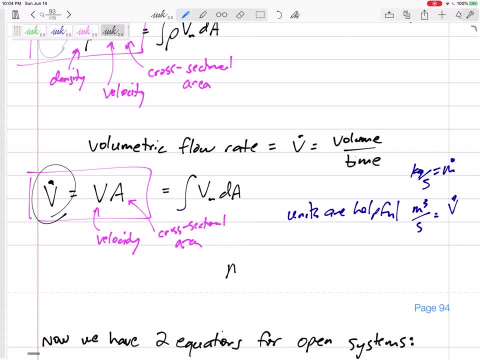 given volumetric flow rate. but you really want mass flow rate. Mass flow rate equals rho, V dot, And again the units would have given that away to you. Here's one more. How about V dot over Specific volume? M dot is also V dot over specific volume. That one, I feel like we've. 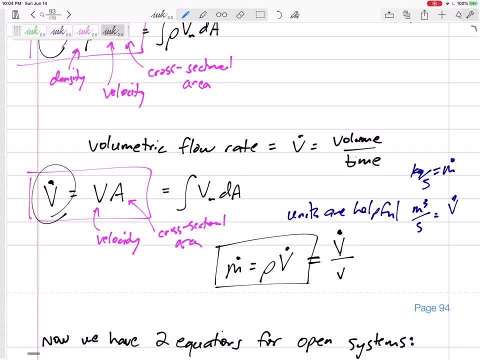 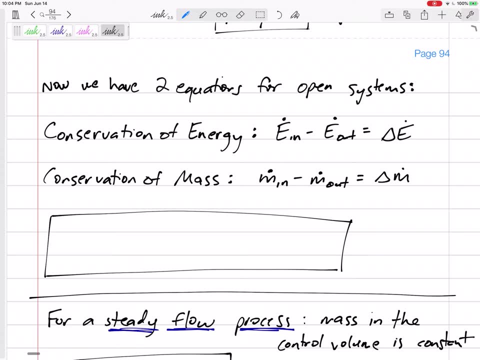 used before. Okay, So anyway, there's some ways to calculate the mass flow rate. Now we've got two equations: the energy in and out. conservation of energy, but also the conservation of mass. It's almost like a new equation- conservation of mass equation. So 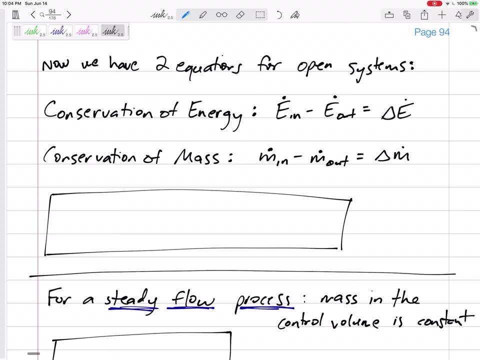 we can talk. think about all the mass. Yeah, So all the mass going in minus all the mass going out equals the change in mass. Or in this one, this is the mass rates. right, That dot is the per unit time, The mass flow rate. 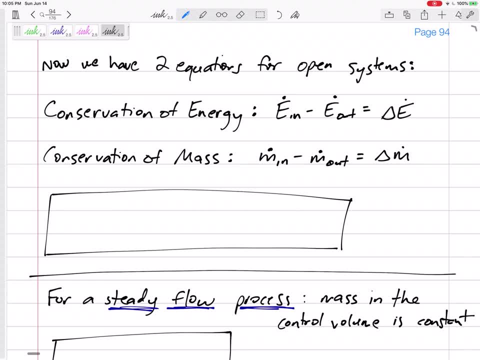 in minus the mass flow rate out equals the change in mass over time. that dot is divided by time. So this way I would kind of think about this and write this: all the rho V A's of the inlets minus all the rho V A's of the outlets equals the change in mass. So I would 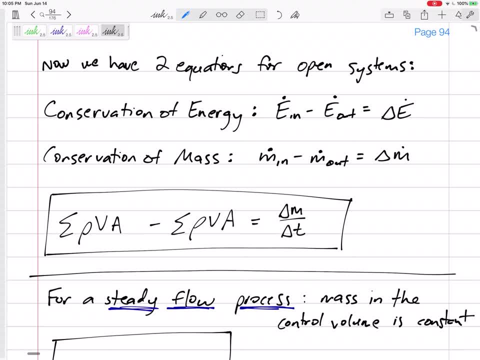 in mass over change in time. if we were doing some integrals and derivatives, this would like be dm, dt, like the derivative of M with respect to time. but most of our we're going to be discrete change in mass and what's the change in time? all right. so we've got the inlets positive, going in the outlets negative. 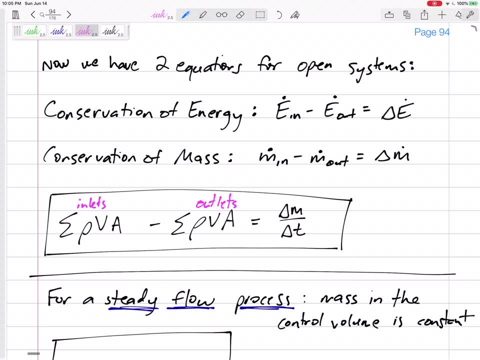 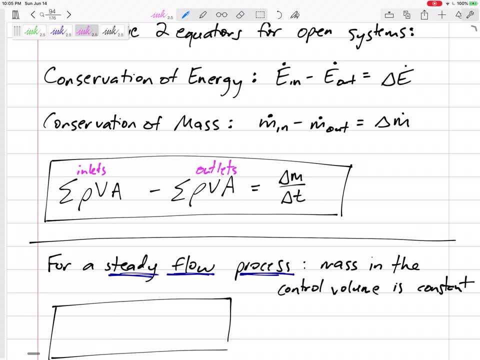 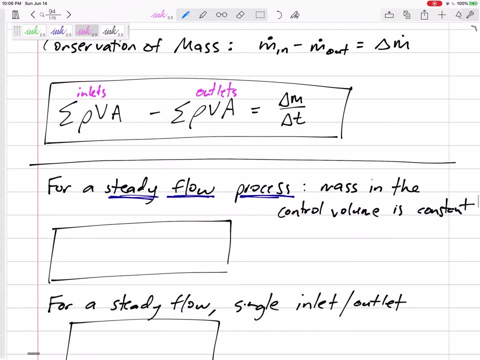 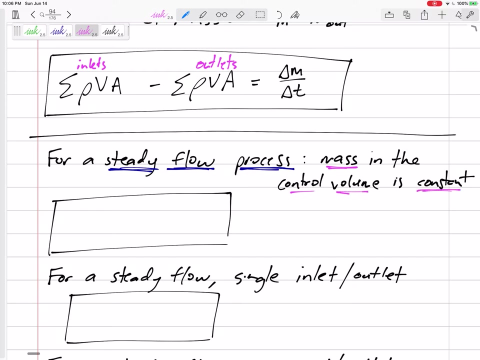 going out. that's how I do everything: everything in is positive, everything out is negative. okay, so for steady flow processes. so first we're going to look at a special type of process and that's a steady flow process. steady flow meaning the mass in the control volume is constant, so it's not filling up with. 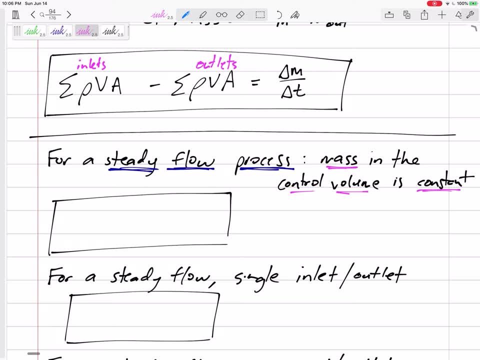 mass. you know, we sometimes I think of inlets, like a hose that's filling up a bucket. all right, that would not be a steady flow process. steady flow processes are not collecting more and more and more mass, whatever mass it started with. that's the master dented with, if the mass is. 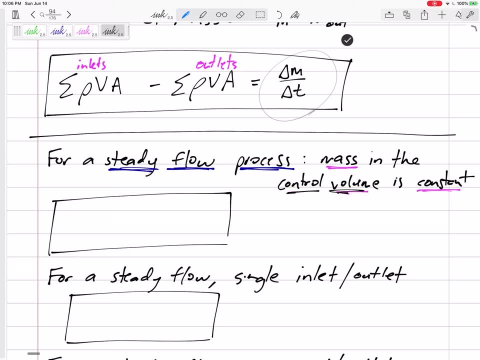 constant in the control volume, then that right-hand side of our equation- delta M dt or dm dt- is zero. and if the right-hand side of our equation is zero- and i'm just going to take this and add it to the other side of our equation, so 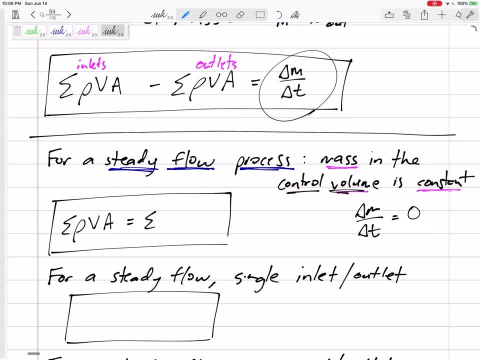 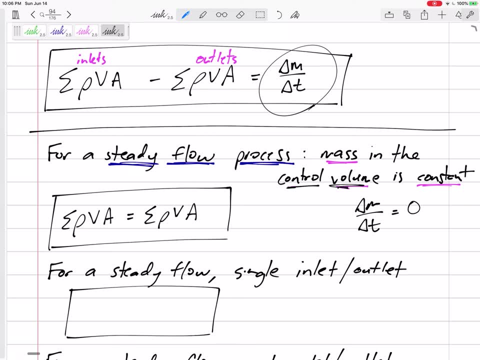 it's really just telling me that all the Equals, all the outlets. So our conservation of mass Becomes that equation right there. The rho VA of the inlet Plus rho VA of this inlet Plus rho VA of this inlet Equals rho VA of the outlet, And that makes sense. 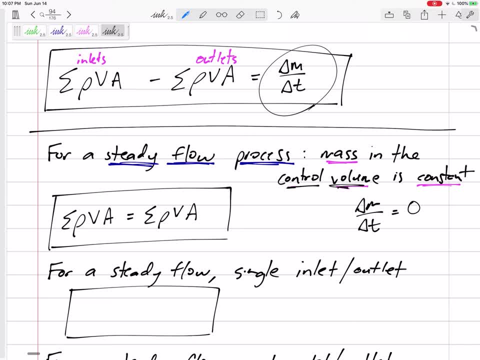 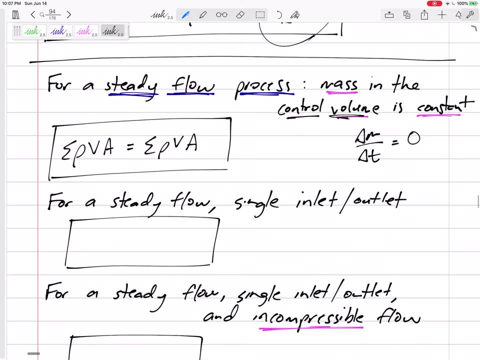 For steady flow devices that aren't collecting any mass. Mass is not changing. All the mass going in equals all the mass going out. That's what it says. All the mass going in equals all the mass going out. If there's a single inlet outlet, Then there's no summation. 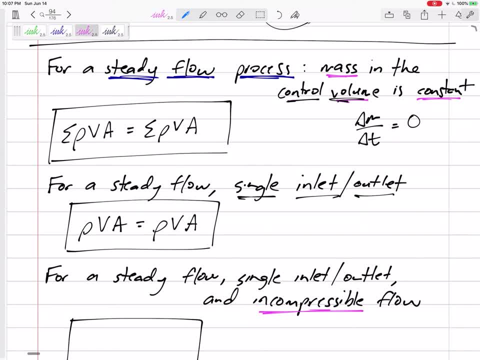 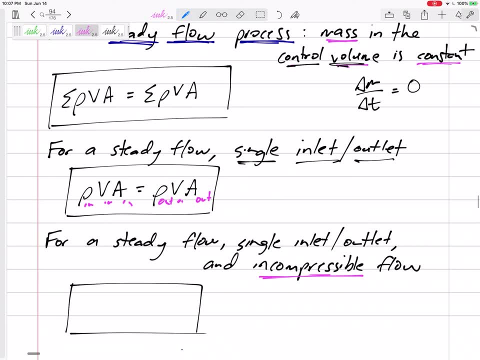 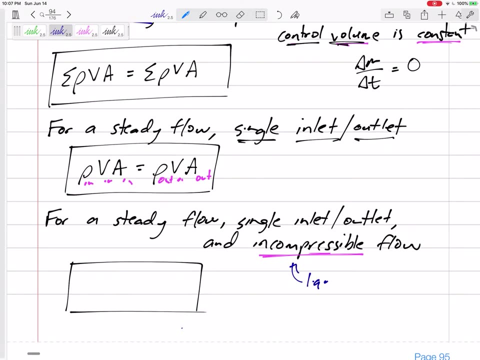 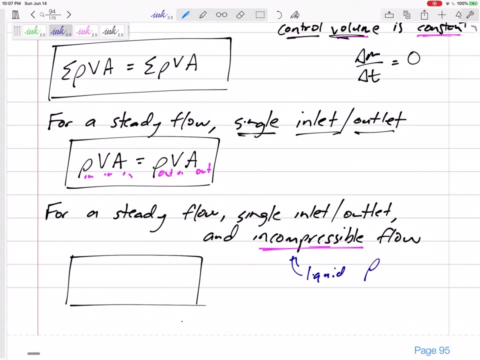 It's just rho VA inlet. I really should say in, in, in, Out, out, out. Now how about steady flow Single inlet outlet And incompressible fluid, Incompressible like a liquid, Not a gas. But if it's a liquid And if we can assume that the rho 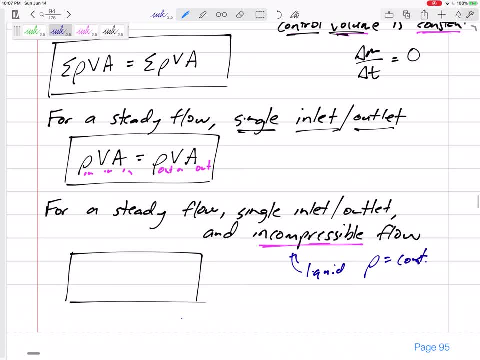 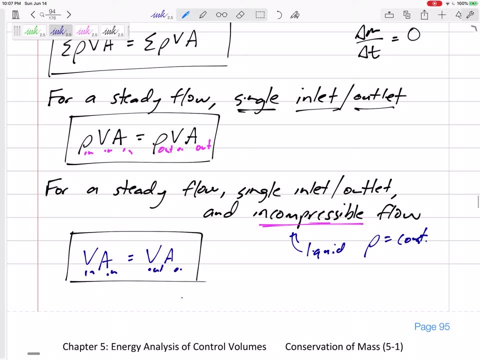 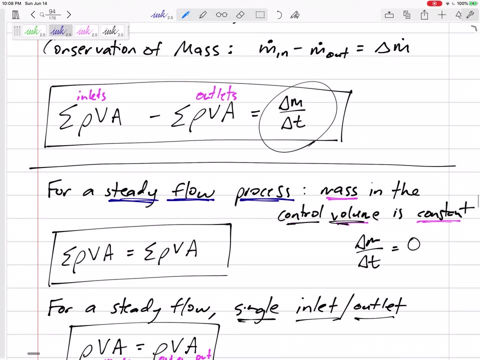 Is constant, Then the VA of the inlet Equals the VA of the outlet Right the inlet, inlet, outlet, outlet. You could, you could put those on your formula sheet, You could memorize those, Or or you could just Well, or you could just start right here.